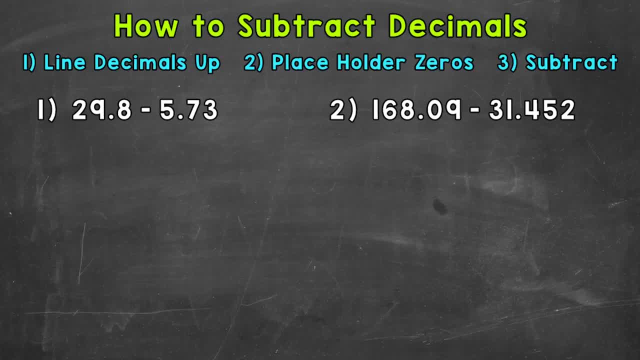 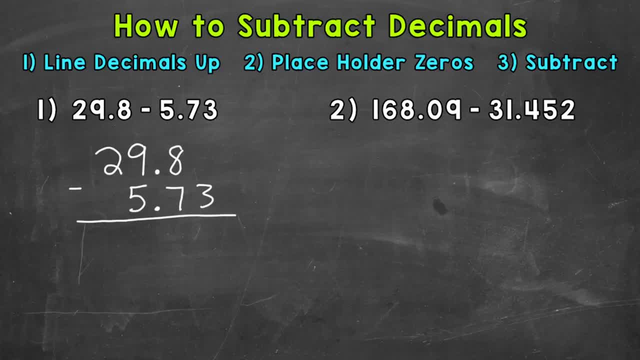 The 5 and 73 hundredths goes further to the right than the 29 and 8 tenths. That's okay. The most important part, we have our decimals lined up. Now, we can use placeholder zeros to make this problem look a little more lined up, meaning we can place a zero in the hundredths place right here. We're using placeholder zeros to better align the problem. Remember, zeros to the right of a decimal do not change the value. That's an equivalent decimal there. So we're not changing the value of that number or the problem overall. Now we're ready to subtract. So we start with 0 minus 3. So we're going to need to borrow. So let's borrow from this 8. And now we have 10 minus 3, which is 7. Then we move to the tenths, where we have 7 minus 7, which is 0. Now bring our decimal straight down. The decimal should be lined up throughout the entire problem, even in the answer. So we place the decimal in our answer by bringing it straight down. 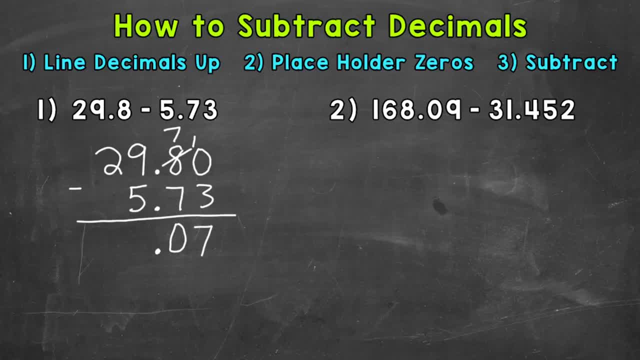 Then we move to the ones, where we have 9 minus 5, which is 4. And then lastly, the tens place, we have 2 minus 0. We don't have anything in the tens place for 5 and 73 hundredths. So let's just bring that 2 down. 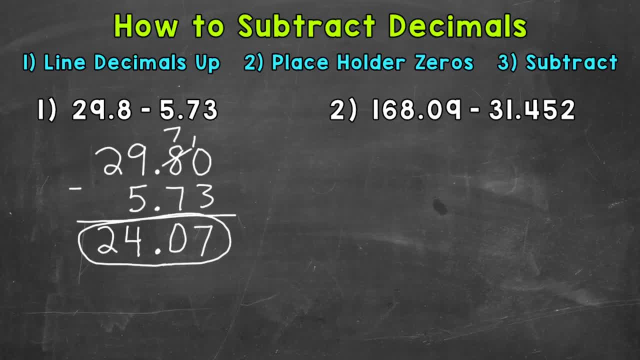 And our final answer is 24 and 7 hundredths. Now before moving to number 2, I do want to mention 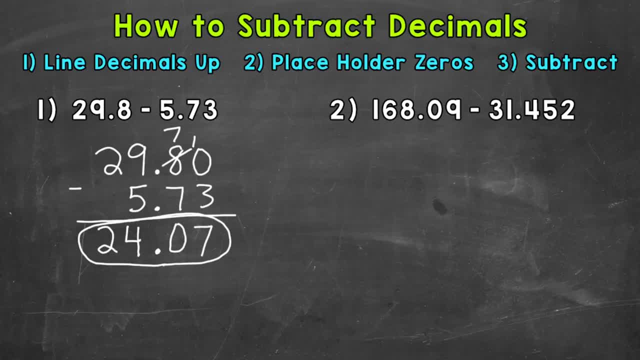 a couple of common mistakes when we subtract decimals. The first one being, let me rewrite the problem here, 29 and 8 tenths minus 5 and 73 hundredths. So the first mistake would be dropping this 3 here, assuming that we can just, drop the 3. But in reality, remember, we have a zero here, and we need to borrow. So don't just drop a number if there is nothing above it. We need to use borrowing, because there is a zero there. The other mistake would be lining the problem up like this. So lining up the digits 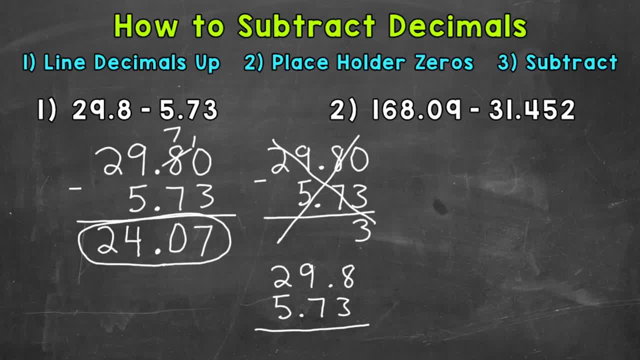 instead of lining up the decimals. So in the case of this right here, you can see that the decimals aren't lined up. We have 3 digits above 3 digits. Remember, line the decimals up. So this will not give a correct answer. Let's move on to number 2, 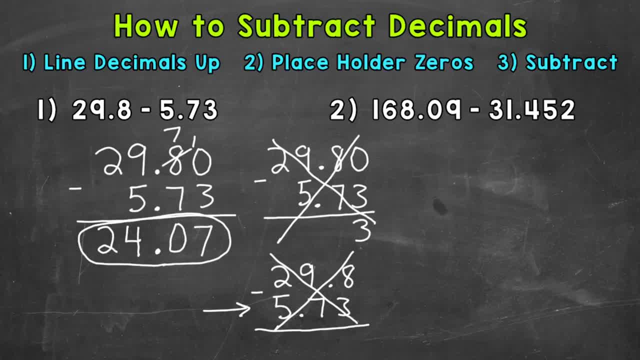 and try another example. So we have 168 and 9 hundredths minus 31 and 452.